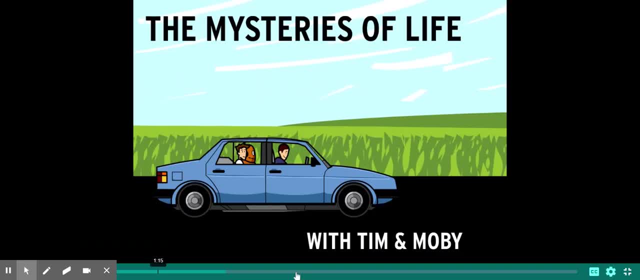 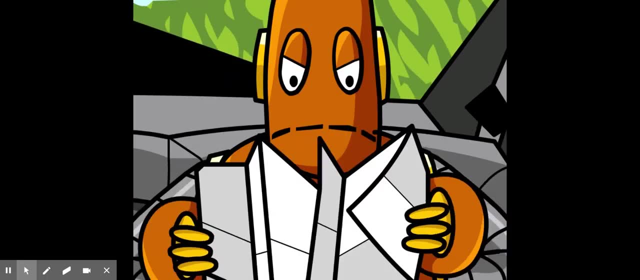 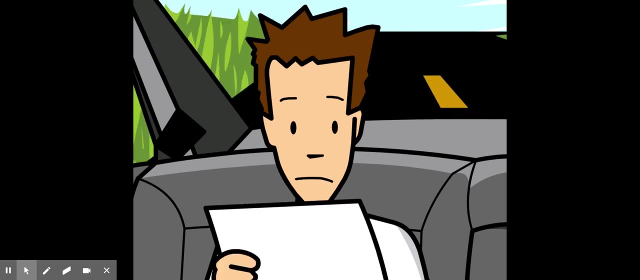 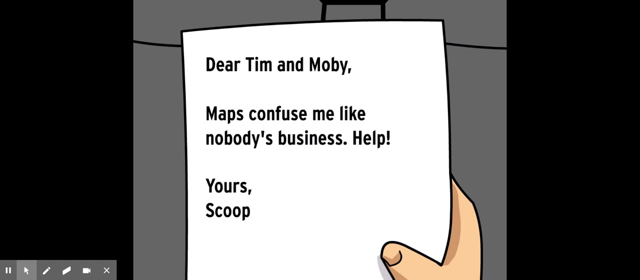 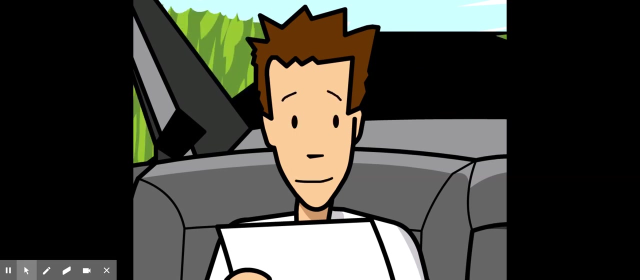 Uh, why don't you let me do that? Hey, that reminds me, Dear Tim and Moby. maps confuse me like nobody's business. Help Yours. Scoop, Hello, Scoop. Moby has a problem with maps too, but they're really not all that complicated. A map is just a representation of some part. 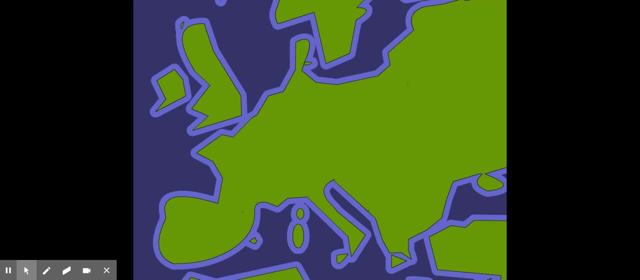 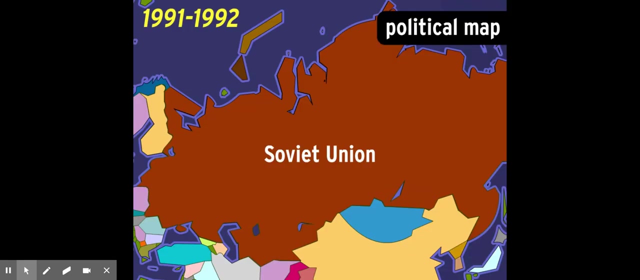 of the Earth's surface. There are all different kinds of maps. Physical maps show natural features like mountains, rivers, lakes, oceans and other parts of the natural landscape. Political maps show borders of areas like countries, states and cities. These can shift. 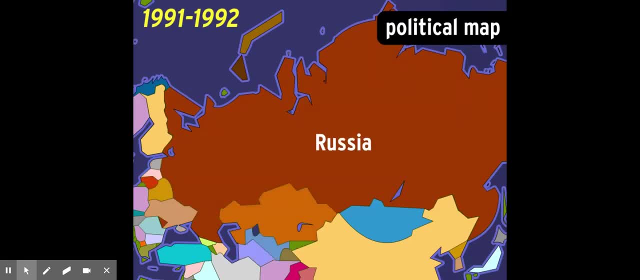 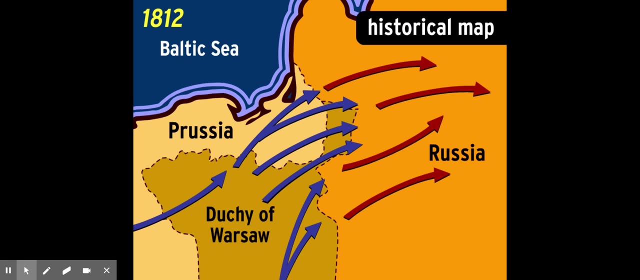 as wars are fought and government changes happen. Historical maps show movements of people, changing borders, battles and other historical events. This one shows the march of Napoleon Bonaparte's army into Russia. The blue arrows represent Napoleon's army and the red arrows 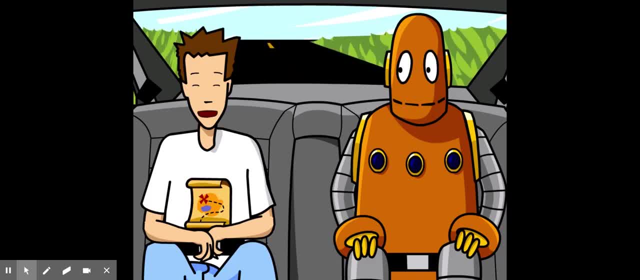 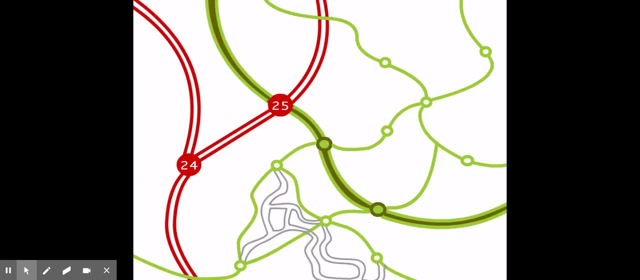 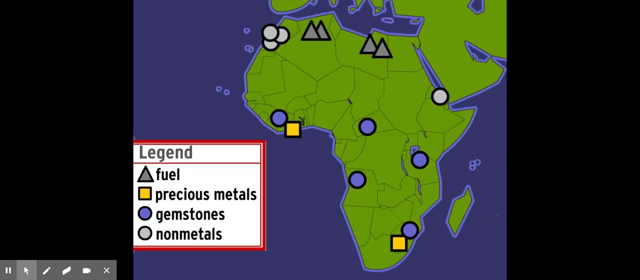 represent the Russian army. There are lots of other types of maps, each with different uses. There are nautical maps, geologic maps, topographic maps and road maps, just to name a few. Most maps, though, have certain things in common. One thing: just about any map will: 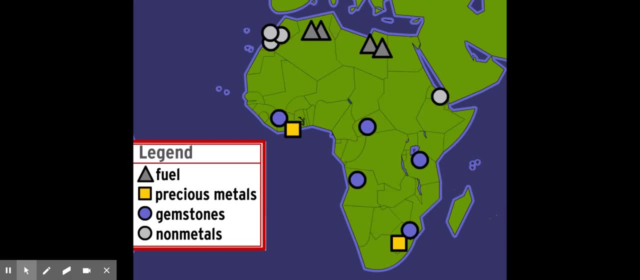 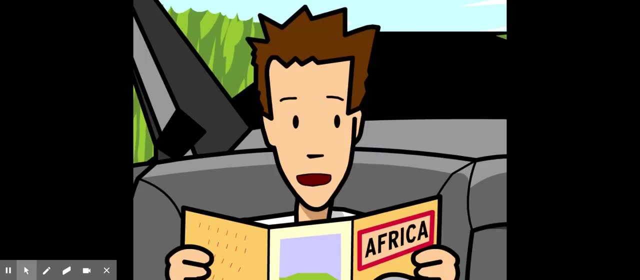 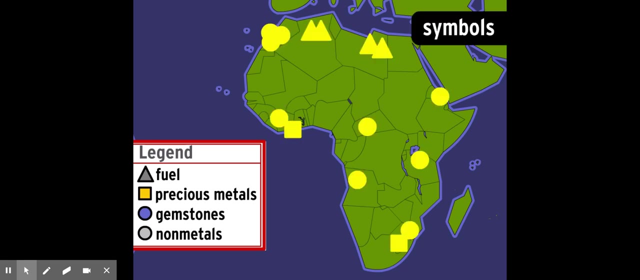 have is lines that show country borders and major rivers. This map shows the mineral resources of Africa. Yeah, you can really make a map of pretty much anything. On this map, colors and symbols play a big role. Symbols are little pictures used to represent anything you want. 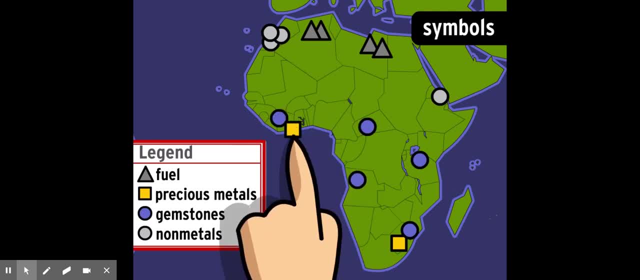 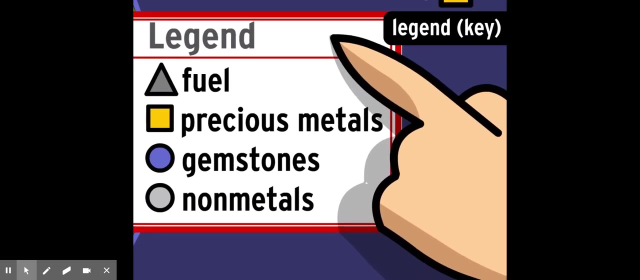 Here: gray triangles represent fuel, yellow squares represent precious metals like gold, blue circles represent gemstones and gray circles represent non-metals. Oh, I just looked at the legend, or key. A legend tells you what the symbols, lines and colors on a map mean. See, this one shows what the symbols. 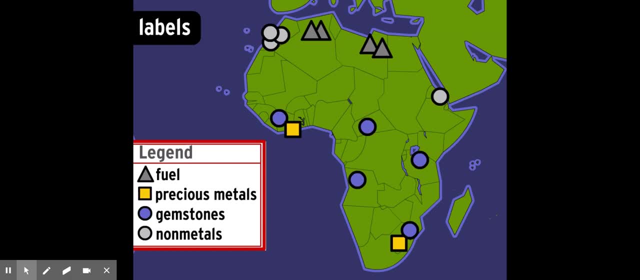 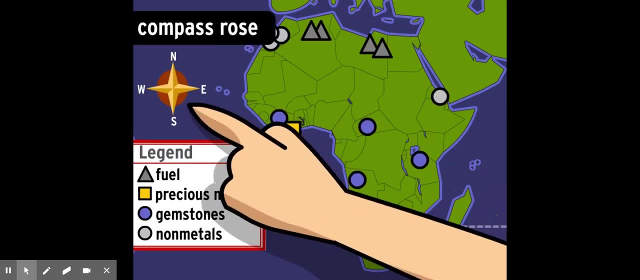 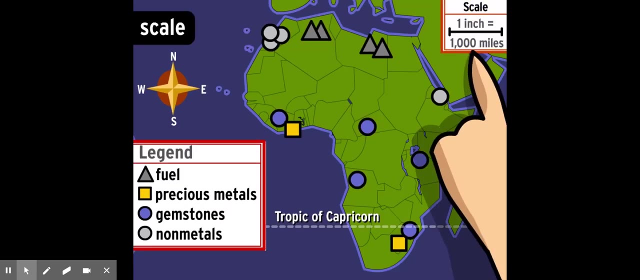 represent. Labels are words that can explain something about the map. This one says Tropic of Capricorn. A compass rose tells you which way the map is shaped: north, south, east and west are, And a map's scale shows the ratio between the distance.